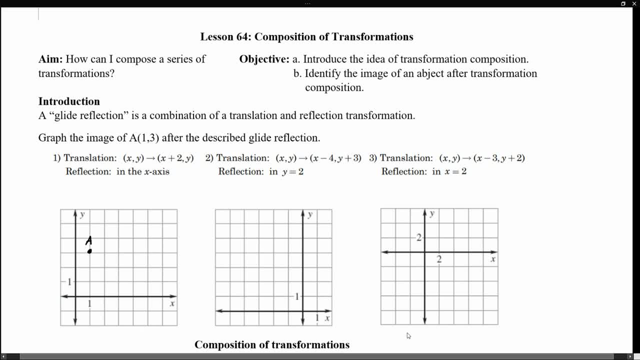 Alright, so let's start by looking at some examples. We'll start by defining what a glide reflection is. A glide reflection, it's a combination of a translation and a reflection transformation. So when we talk about glide reflection, we're talking about performing two actions on the object. 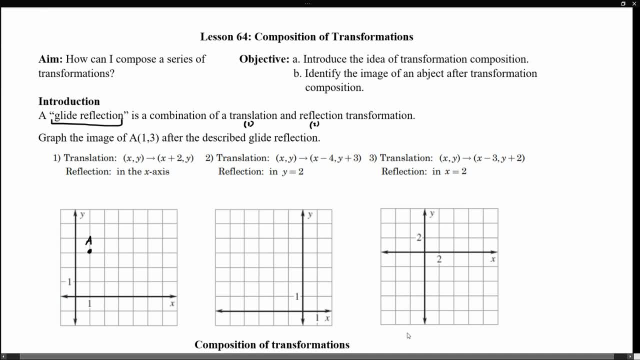 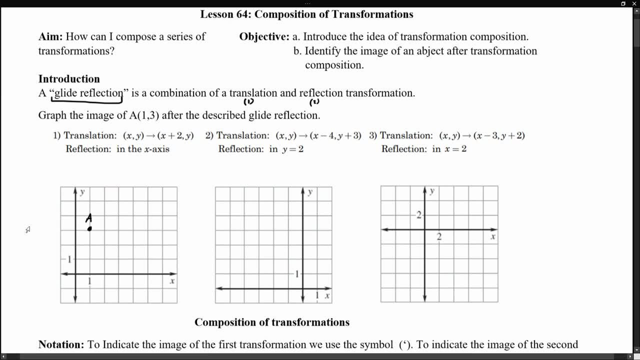 A translation and then a reflection. So how does that exactly look like? Well, let's take a look at example one Here. Let's start by plotting the point A, which it's already done here for us at 1,3.. 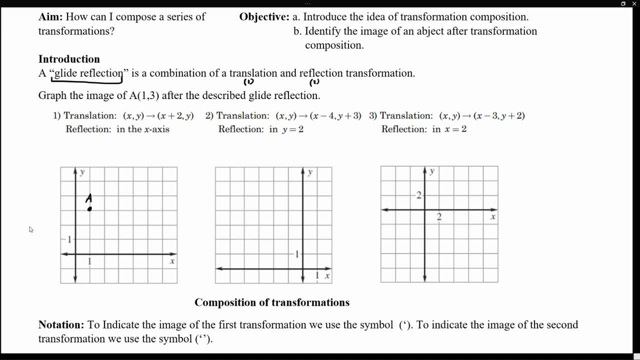 And let's perform the glide reflection. So first let's perform the translation. So let's understand the notation. The notation here says: look, get a coordinate point X and move it two units to the right. So A, if we move it two units to the right, is going to be right here. 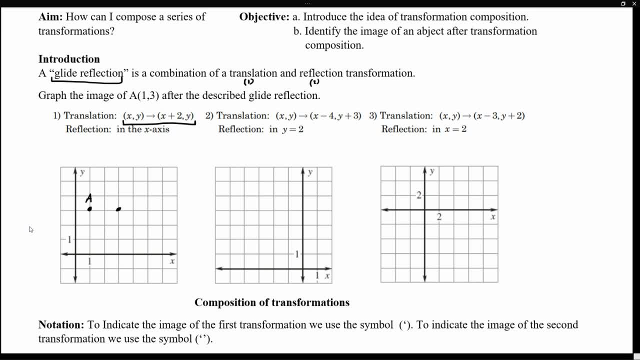 And notice that I'm only moving it two units to the right Because Y it gets mapped to Y, So the Y doesn't change and the X gets moved two units to the right. If this would have been a subtraction, then we would have been moving two units to the left. 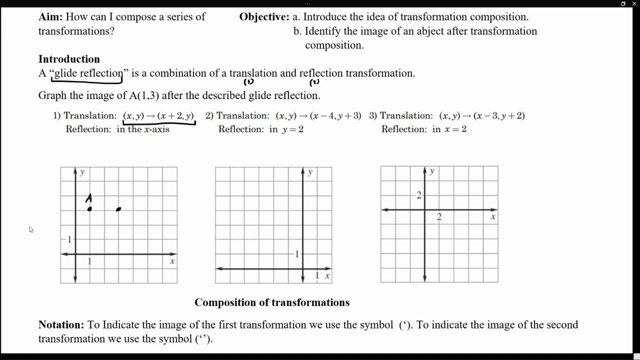 So notice that we have done one transformation. So therefore, this point, right here, we want to refer to it as A, with one prime on it. So that is just saying I have performed one transformation on A. Okay. Okay Well, since we're doing a glide reflection, we've got to perform two transformations. 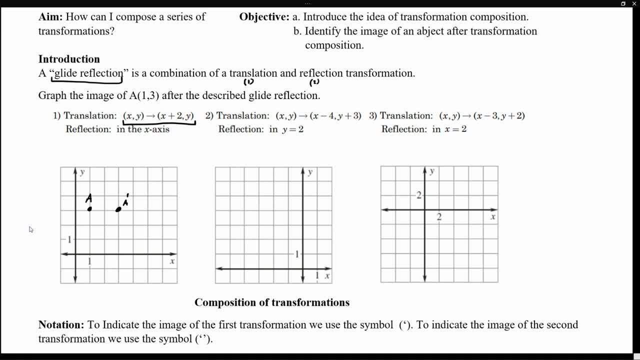 So translation it's already done. So now let's reflect our image. But now we've got to be careful when we're doing this, because we're not going to reflect the original, but we're going to reflect the image of what was given. 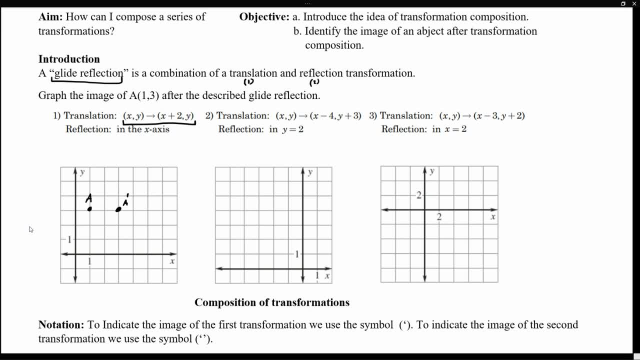 So let's reflect A And again remember that one of the properties of reflection is that the point should always be equidistant to the line. Okay, So now we're going to reflect the image of reflection. So what is the line of reflection that we're interested on? 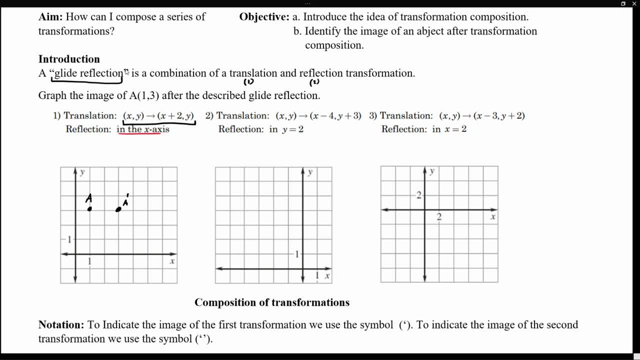 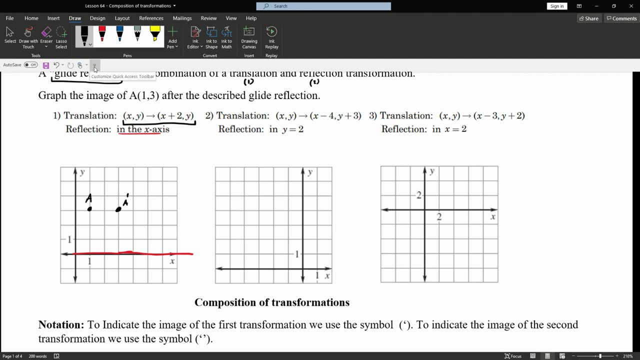 The line of reflection that we're interested on is the X-axis. So here we have our X-axis, So let's just reflect this object. So if this is A prime, and we reflect it well, A prime is one, two, three units away. 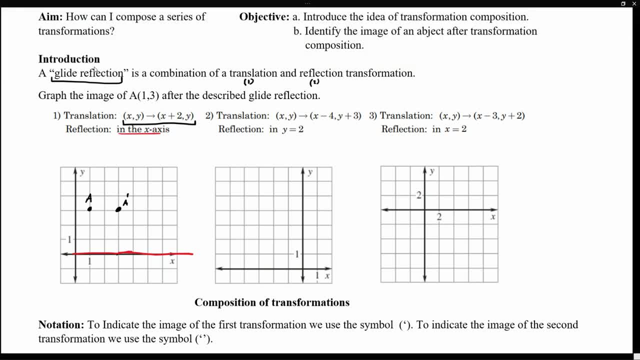 So therefore, after performing this reflection, it should still be three units away. So we go one, two, So the product of that reflection should be somewhere down here. Well, let's be careful with the notation now, because now this point is the result of performing two transformations. 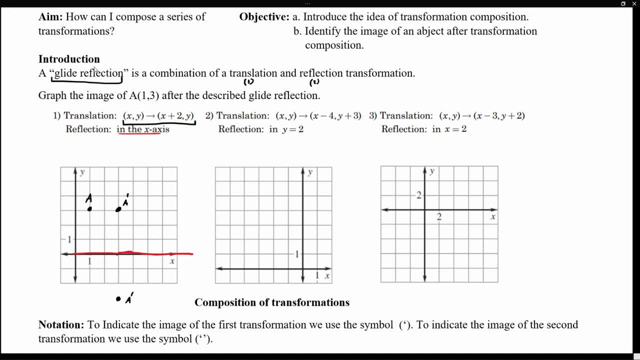 So therefore this point: it will be considered as A prime prime. So it's not that clear there, So let me just rewrite it one more time, Because A prime prime, Every single prime That we put on top of a letter. 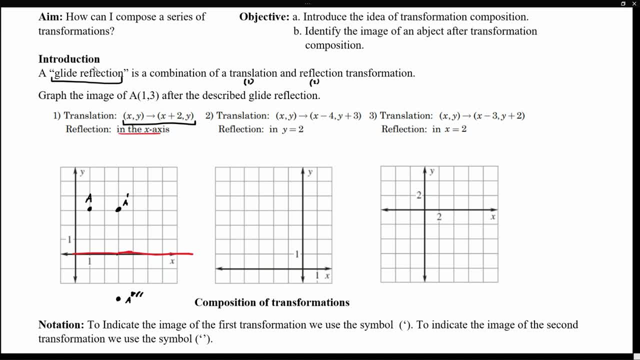 That indicates that that's the image of how many transformations that we have gone. So notice that this point down here is the product of performing two transformations. My first transformation was a translation and then I reflected, So therefore this point is the product of two transformations. 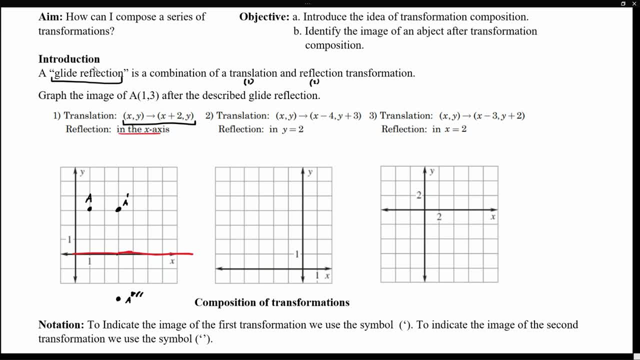 Therefore it should have the notation of A prime, prime And again, composition is just the idea of Performing more than one transformation of an object. Let's perform another glide reflection, real quick Still. let's start by still putting a recording, a point at one comma three. 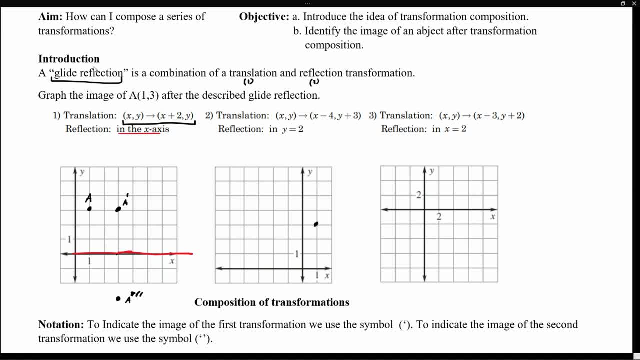 So one comma three. So here we have our A, just like we have it here. Now let's perform this translation. What this translation is saying: Look my X values- I'm going to move it for units to the left- And also my Y values. 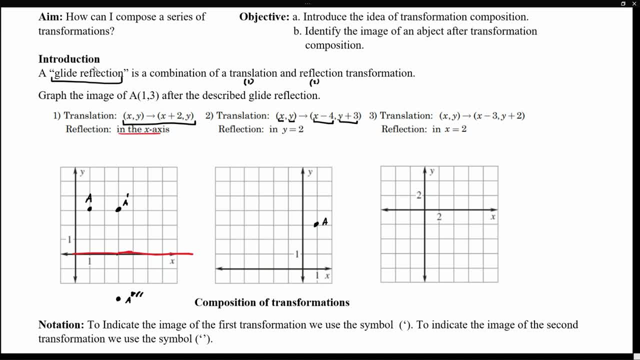 I'm just going to move it three units up. So let's take a look at A, and at A we're going to move four units to the left. So one, two, three, four and three units. So one, two, three. 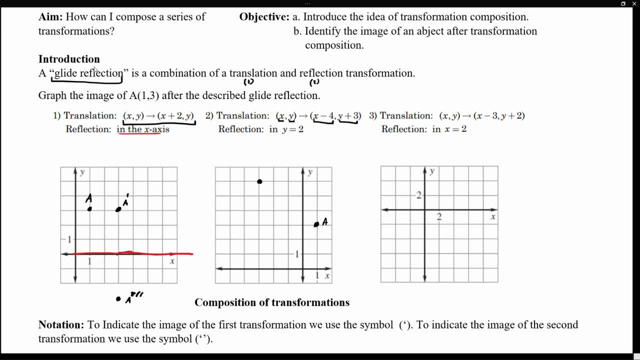 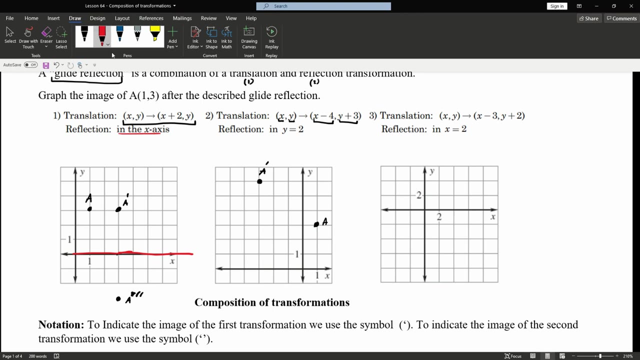 So notice at this point- is the product of performing a translation. So therefore this point is considered as A prime. Now let's perform a reflection on the line Y equals Two. Well, Y equals two. It's essentially this line, right here? 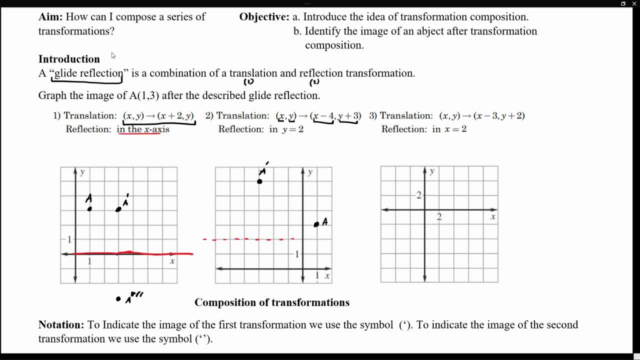 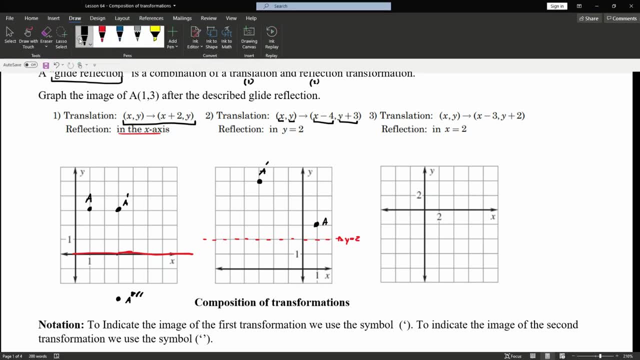 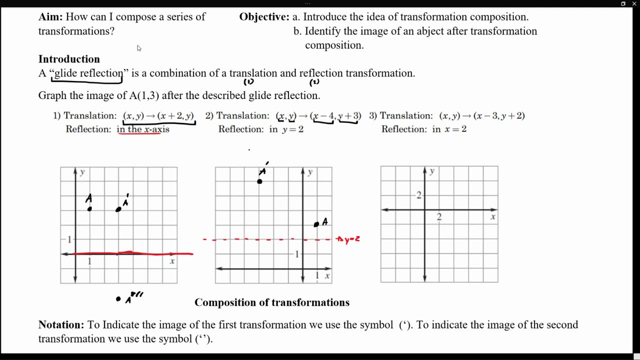 So let me just do it in dotted. So this dotted line will represent the line. Y equals two. So let's just reflect, Let's just reflect our A prime point. So we want to reflect it with this line. I know that the distance should remain two. 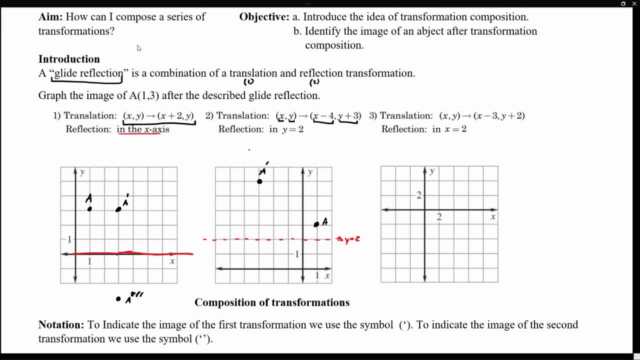 So if A prime is one, two. One, two, three, four units, Then the reflection should be four units away from the line as well. So that would be one, two, three. Let's just say that it's somewhere around here. 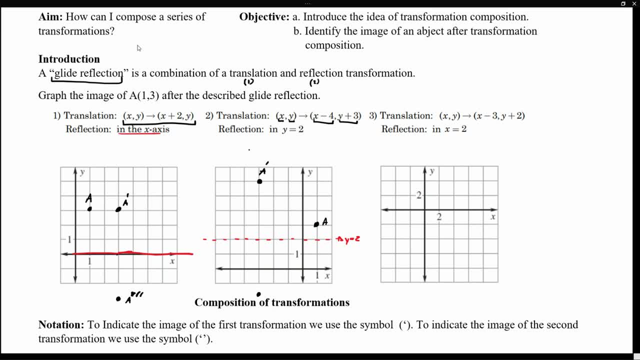 And notice at this point, it's the product of performing two transformations, So therefore this point should be labeled as A prime prime. We perform one transformation, That's A one prime. We perform a second transformation, So that's A prime prime. 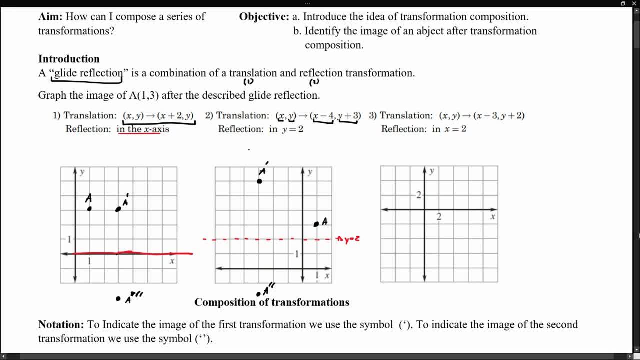 So let's just perform one more light reflection, just to be sure that we're okay with it. So again, let me just choose the same point, One comma three. So I guess you just got to be careful here, because now every square has a unit of two. 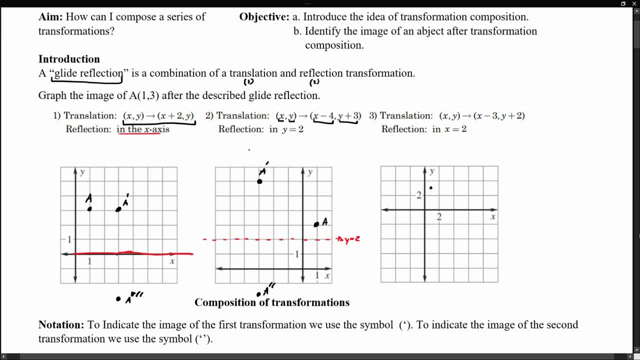 So that's one comma three. So that's somewhere around here. That would be A, And again, let's perform our. Let's perform our translation. This is saying that X is going to get moved three units to the left and Y is going to get moved two units up. 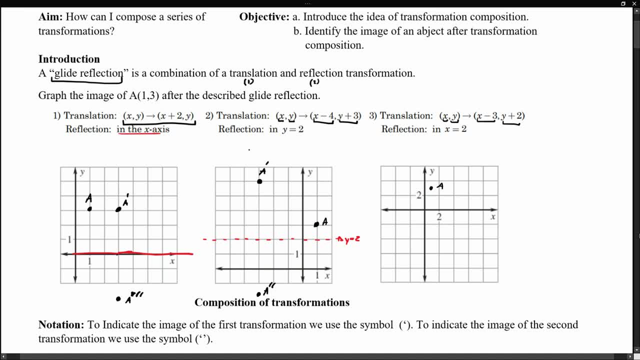 So let's get our point A and let's perform that translation. We're going to get A and we're going to move it three units to the left, So that will be one, So that would be around here, And let's move it two units up. 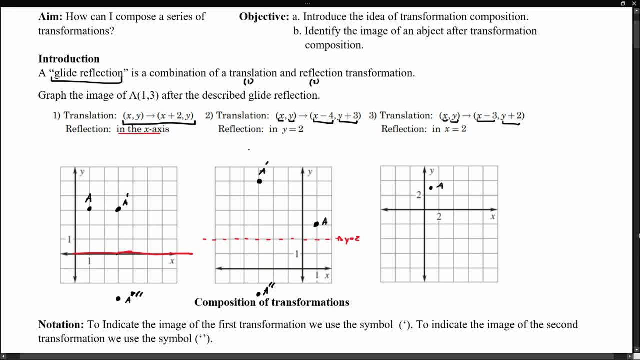 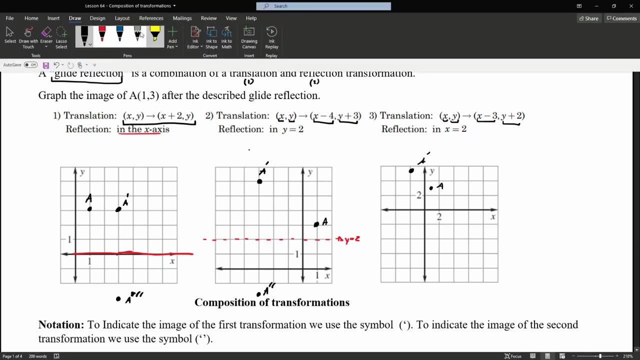 And again, every square it's two units. So that should be somewhere around here. So this will be considered my A prime, since I have only done one transformation. Let's perform the reflection over the line X equals two. Let's see where is X equals two. 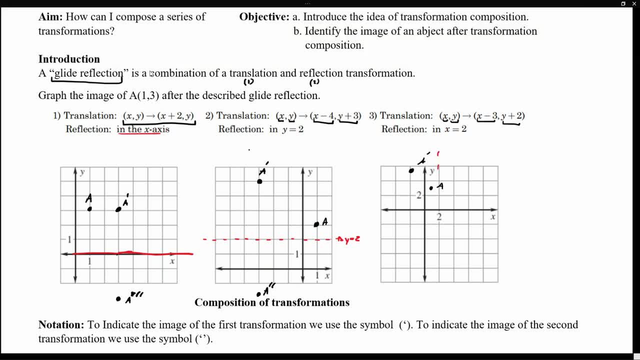 Well, X equals two. It's this vertical line right here. So let's just perform our reflection. So notice that this point is four units away from X equals two. So therefore, after performing our reflection, it should still be four units away. 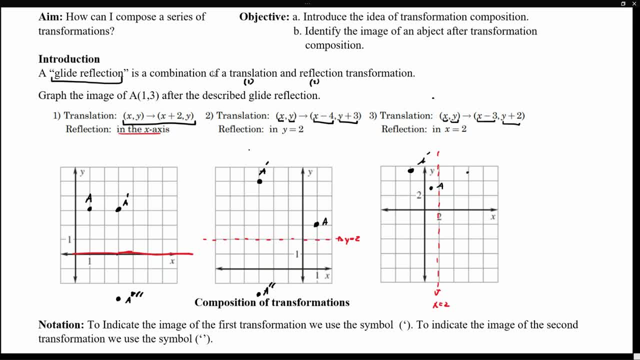 So that would be one, two and that would be four right here. So now notice, at this point this was four units to the right. So after performing the reflection, that should still remain still. So now, at this point, exactly right here, this is where A prime prime is located at. 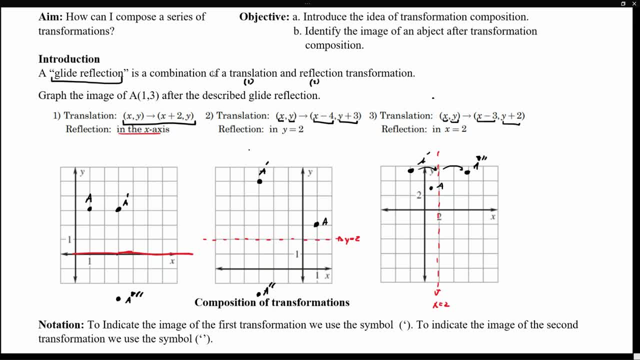 So these examples were, more than anything, for you to just get comfortable with the notation And for you to get comfortable with the idea that we can perform more than one transformation of an object. And right now we're just doing a single point. We're going to move on to the next one. 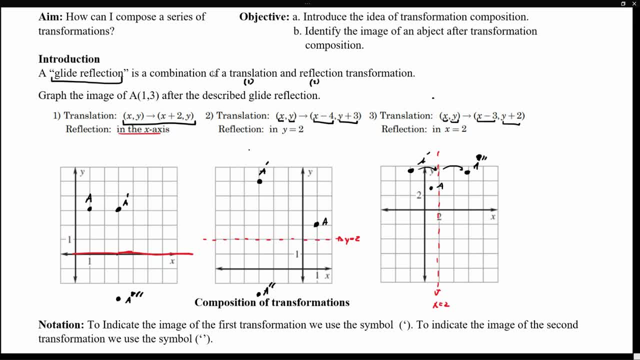 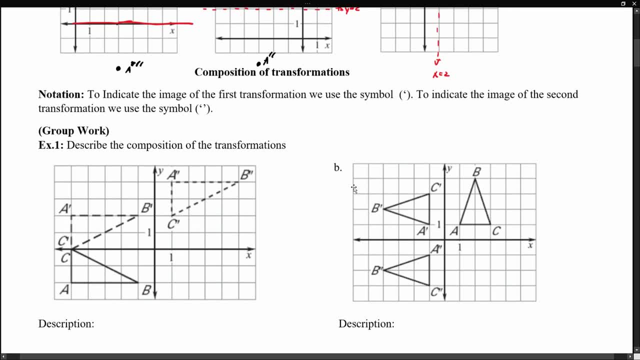 Full objects in a second. So now let's just recap some of the notation. Let's just recap some of the notation. Well, this is a very important notation right here, Because to indicate the image of the first transformation, we only use a single prime. 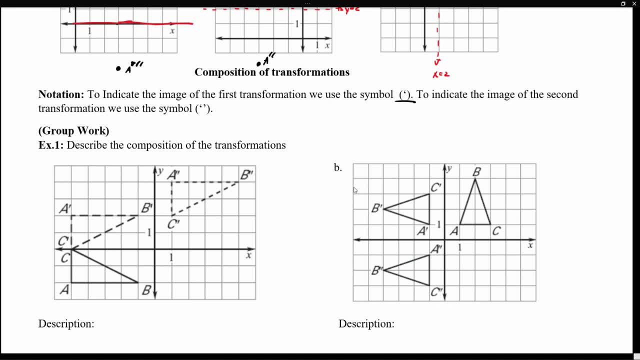 So pretty much the primes are this little symbol that we put on top of letters that indicates the image of what transformations. If you perform two transformations, then we do double prime. If you perform three transformations, then that's A triple prime, And so forward. 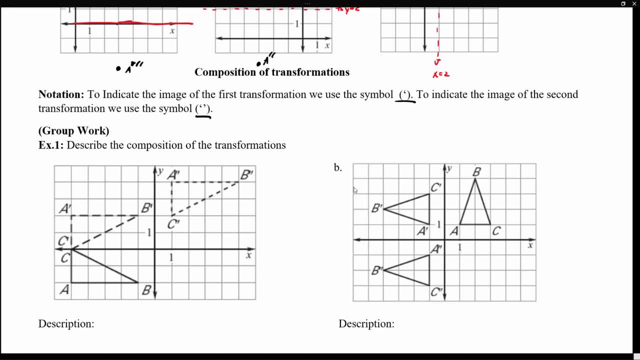 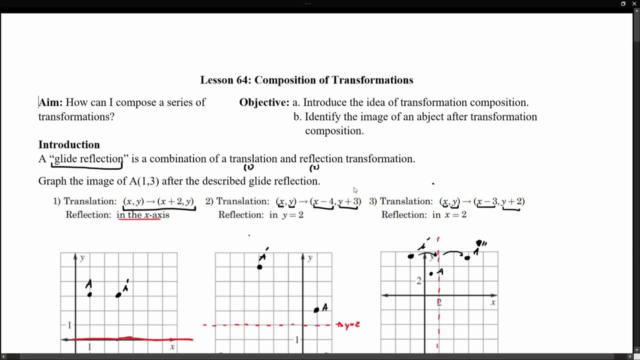 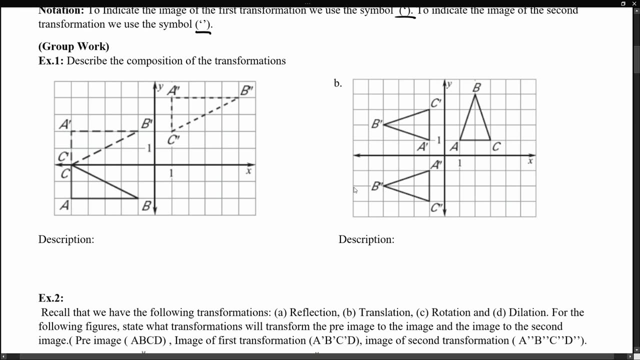 So, even though these examples are labeled as group work, I do would like to go over some of them So you feel comfortable with this concept. Oops, So let's start by looking at example one which says: let's describe the composition of the transformation. 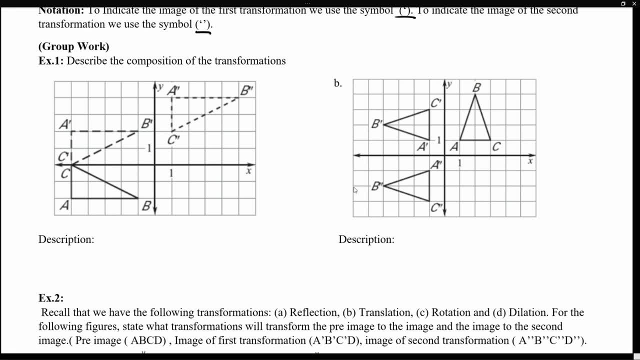 Notice the word composition. So this means that we are going to be doing more than one transformation of an object. Let's let's take a look at how the image is presented to us. So here we have. let me do highlighters, because highlighters are good. 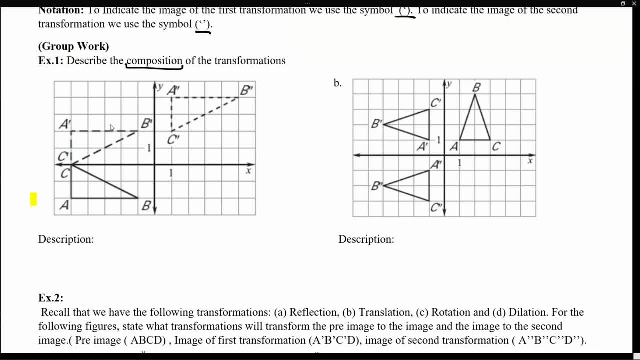 So this is: notice that just by looking at the notation, this is too much. Notice that by just looking at the notation, this triangle doesn't have a prime anywhere. So that's just A, C and B. There is no prime on top of it. 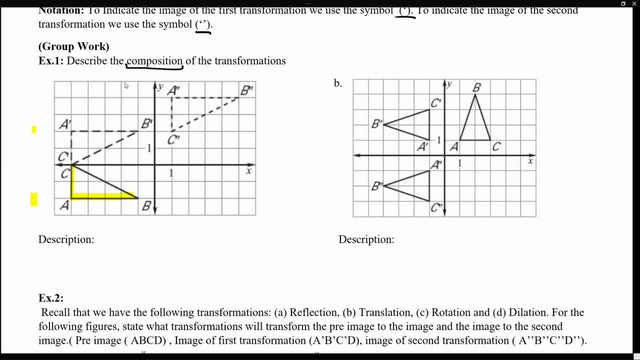 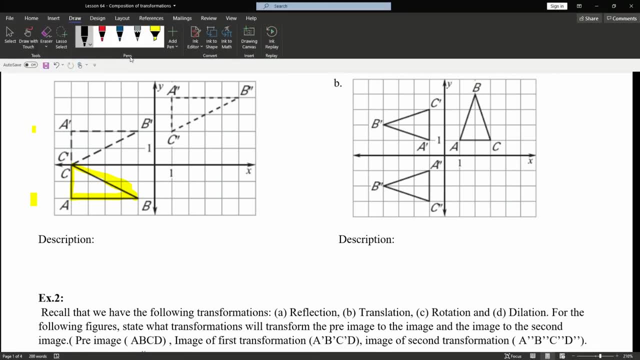 So we can think of this as the original image. This is the original image because there is no prime on top of it, So that means that this is the object that we start with Now. notice that the triangle on top of it, this dotted triangle right here. 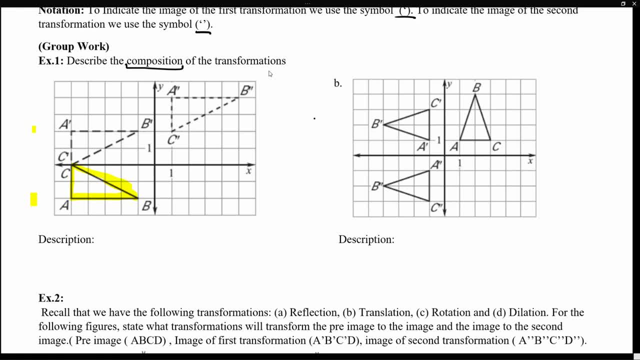 They all, all those letters, have one single prime on top of it. So that's an indicator that this is the first image. So the question now becomes: what can we do to this triangle So it actually lands on top of this dotted triangle? 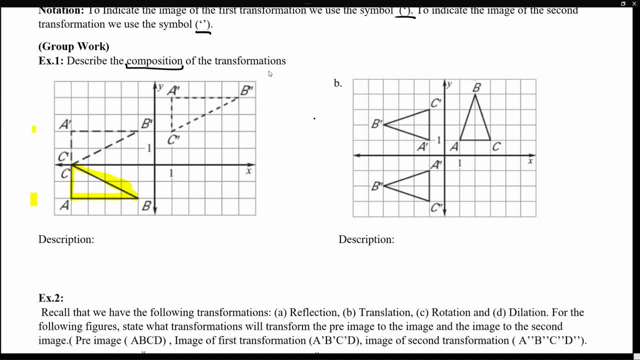 Well, notice that if we get every single point And we reflected over the line, over the X axis- Because let's just take a look at this X axis- If we reflected this triangle over the X axis, notice, at this point, C is going to go to C. 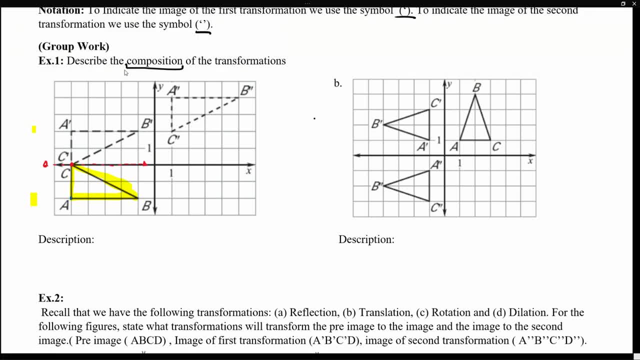 But now this A, it's two units away from the line of reflection, which is also two units away after the line of reflection. So instead, if we get A and we reflect over this line, it's going to land on top of it here. 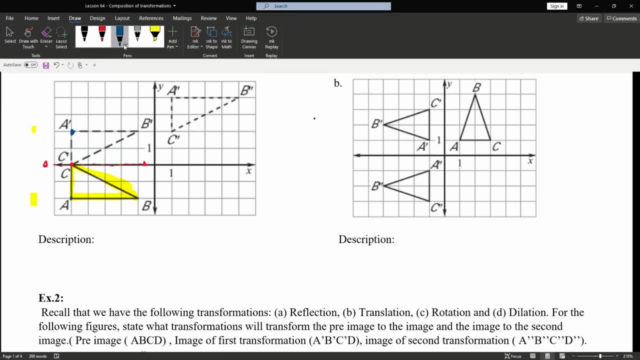 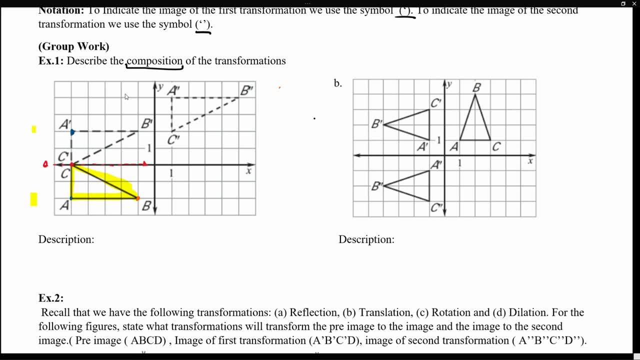 And the same can be said about B. The same can be said about B. Here we have B, And if we reflect it, or if you get the subject and you just flip it along this line, Notice at this point it's going to land exactly at this point. 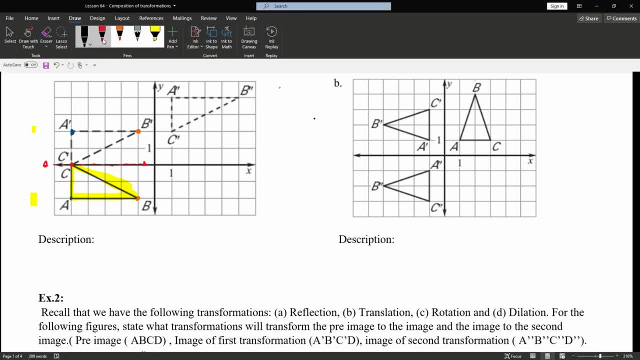 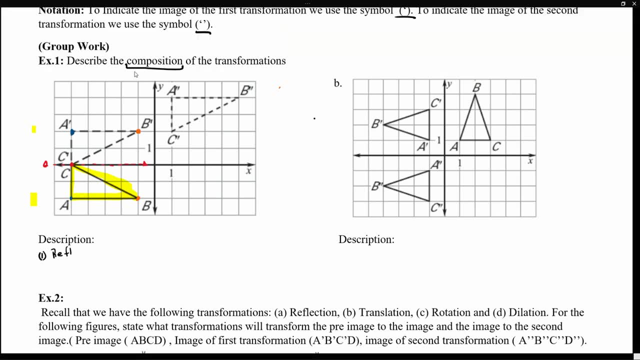 So the first transformation that we did, The first transformation that we did, we perform a reflection Over the line. what would this be? Y equals zero, which is another way of saying- is the X axis. So that's the first thing that we did on this object. 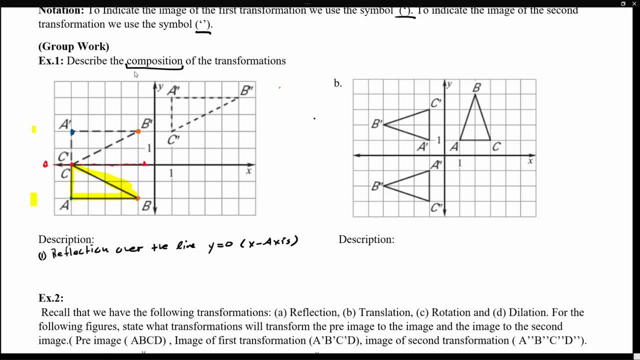 So now the question becomes: what can we do to this image now? What can we do to this triangle so it moves? Or, I'm sorry, I think I already gave it away- But what can we do to this triangle so it lands exactly on this second triangle? 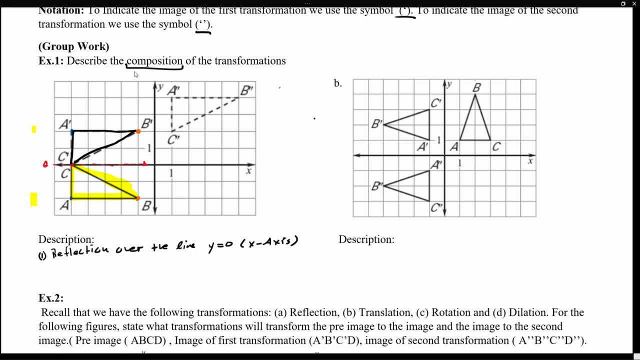 So the first thing you might notice is that it's definitely not right, It's definitely not a reflection. It's definitely not a reflection, But notice that it has the same orientation here. So you can just think about getting this triangle And it seems to just be a solid movement. 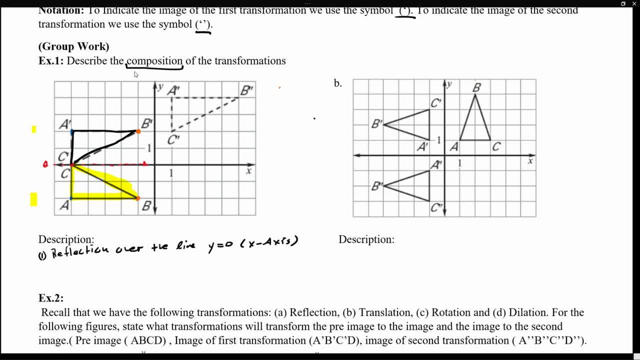 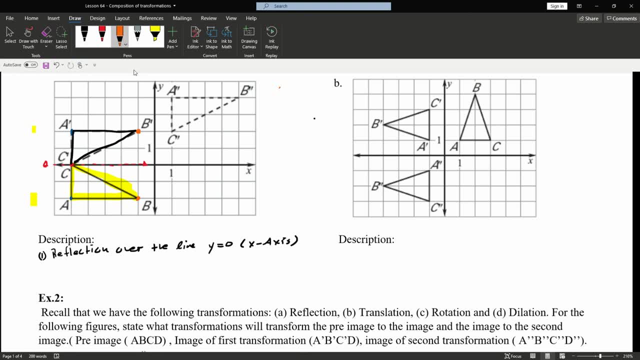 But now let's think about by what units. Let's think about what units are we moving this triangle? Well, triangle A- I'm sorry point A prime. How many units do we need to move it? so it goes all the way to A prime prime. 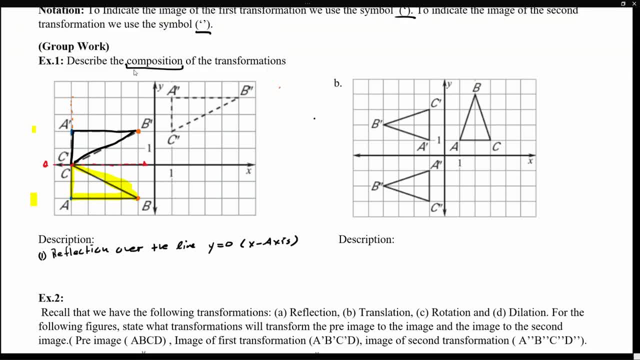 Well, that would be. That would be two units up, And that would be one, two, three, four, five, six to the right. So two units up and six to the right. Now, does every single point in here has the same movement? 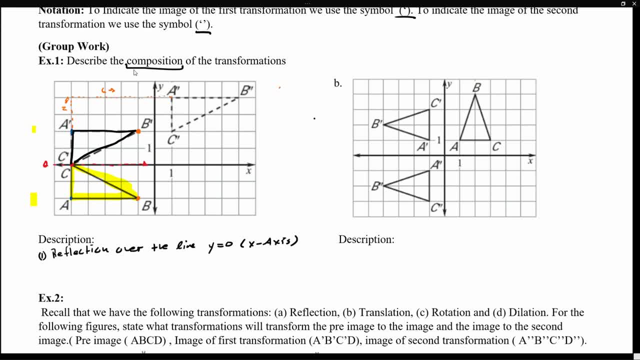 Well, I don't know. Let's see From C to C: prime: two units up and one, two, three, four, five, six. So it lands there as well. B: two units up, One, two, three, four, five, six. 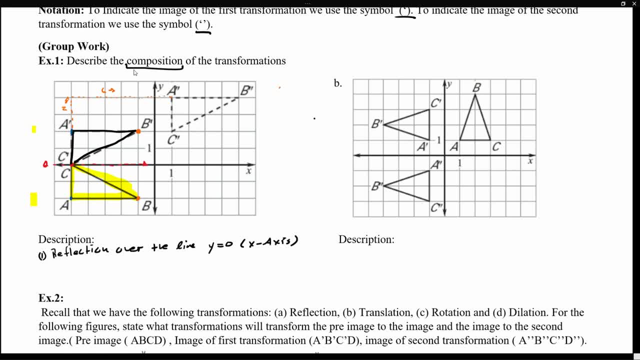 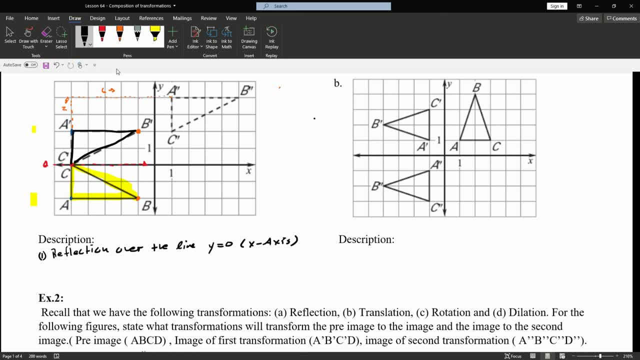 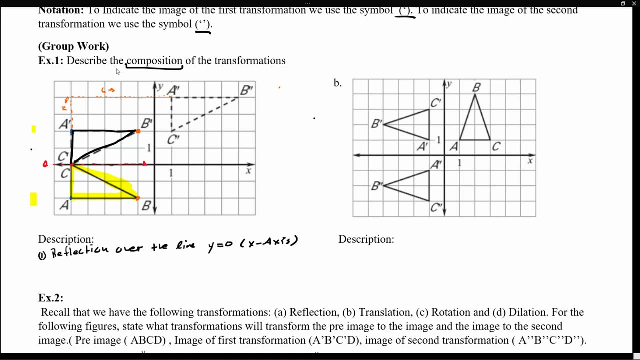 So notice that it works out. So what we have done now is that first, the original object, we reflected over the x-axis, And then we shifted, or we translated, the triangle two units up and six to the right. So the first thing that we did, we reflected over the line y equals zero, which is the x-axis. 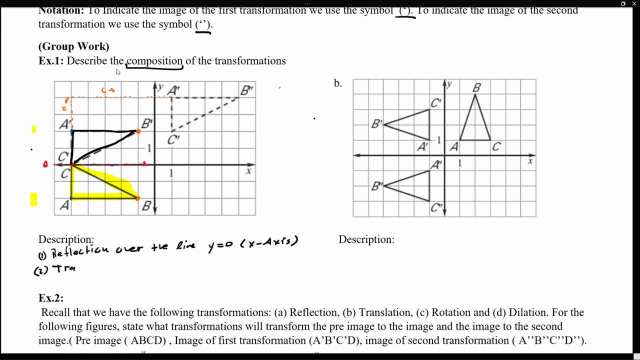 And then we translated the object. We translated triangle A prime, B prime, C prime, two units up and six units to the right. So that's all we're doing. We're just applying the same thing. So that's all we're doing. 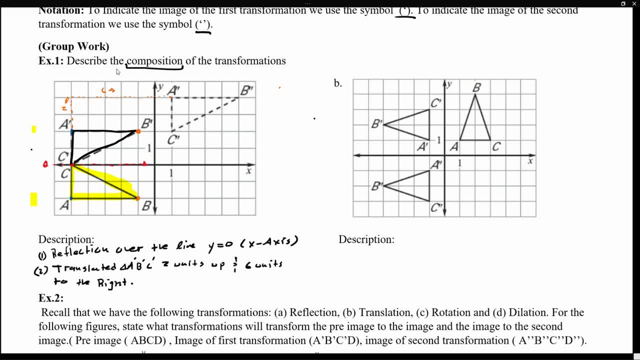 We're just applying different transformations. We could have moved that object even one more time. When we talk about composition, we're not just restricting ourselves to just two transformations, But in this example, we're just doing two. All right, Let's take a look at example two now, or example B. 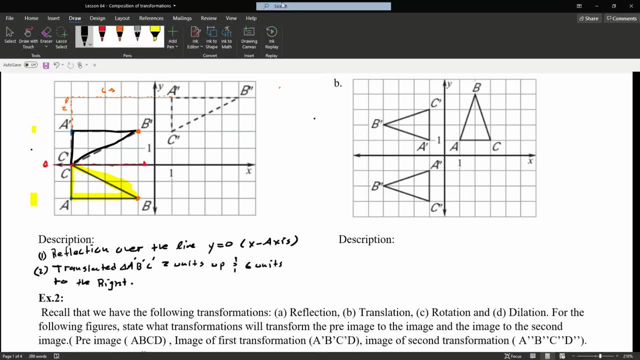 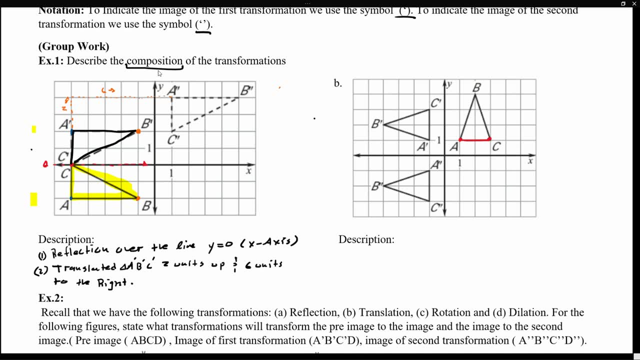 Let's think about this for a second. The first thing you want to do is identify the original image, which in this case, it's right here, Because notice that this triangle doesn't have any of the original images. It doesn't have any of the prime. 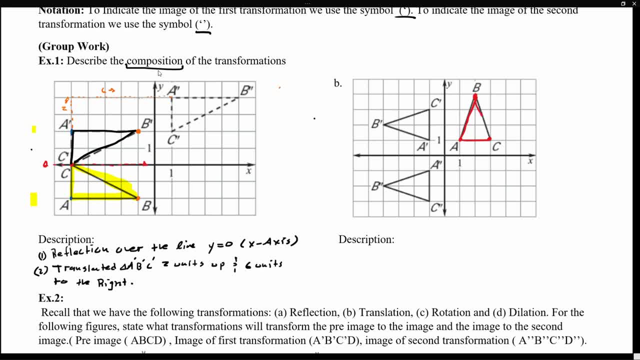 So this is just saying that this is the original preimage. And now let's think about this for a second. What exactly did we do to this triangle So it lands not in this triangle? because notice that this triangle has C prime prime, A prime prime. 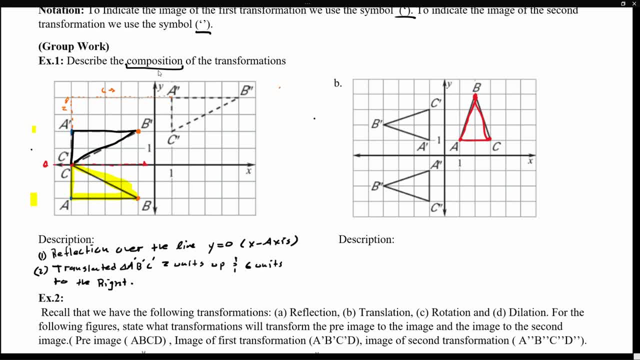 So that's double prime. We want to first land it in single prime. Well, it's definitely not a translation, because if we get this object and we shift it, it definitely is not going to look like this. Is there a reflection? Well, if we get this object, 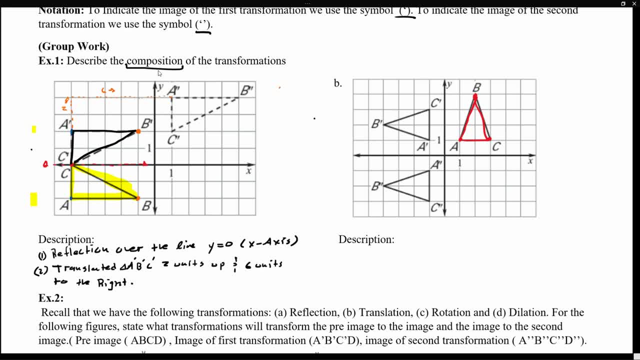 And we reflect it. It should look something like this somewhere around here, just like I'm doing with my cursor. So it's definitely not a reflection. So what is it exactly? Definitely not a dilation. It seems to be the same shape. 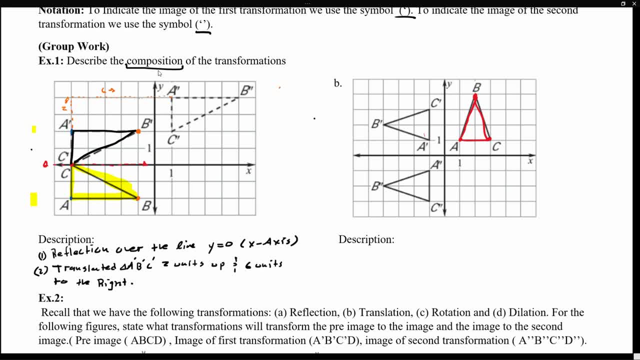 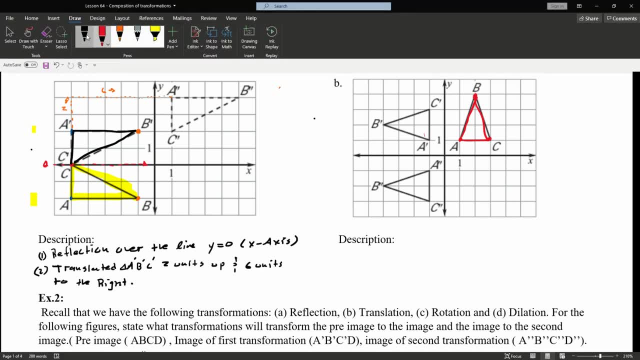 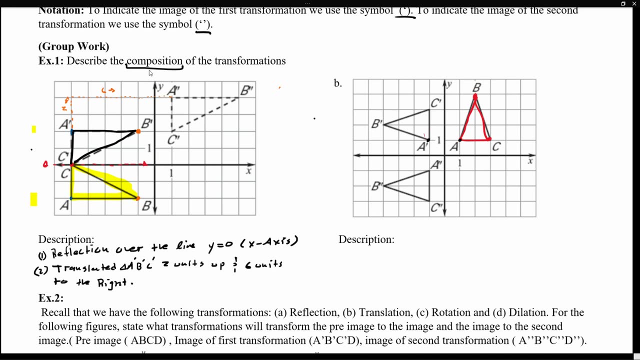 So it must be a rotation. But now, how many degrees are you rotating this figure? Well, let's take a look. We can figure that out, because now this point is one comma one And this point is negative. one comma one, So A is one comma one. 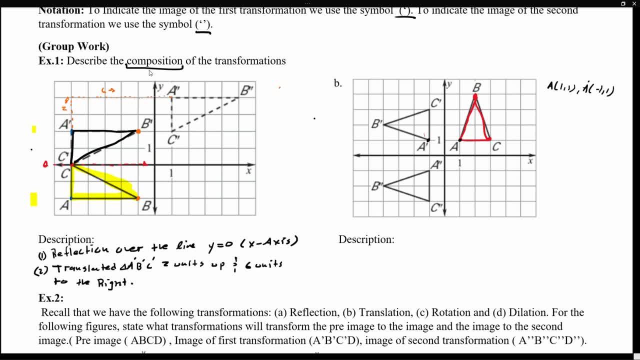 And A prime is negative, one comma one. C is one two, So that's three comma one. Where C prime is negative, one comma three. And I feel like at this point you can start seeing the change. Just remember that when we reflect over the origin, 90 degrees. 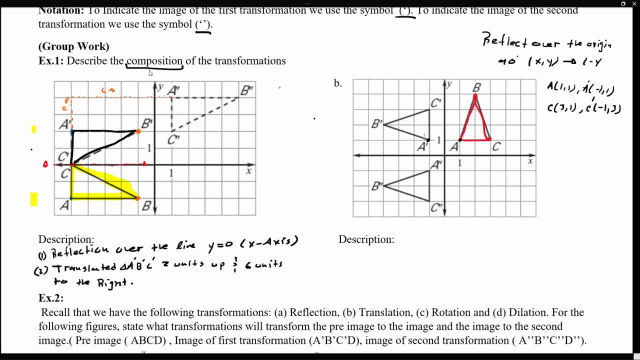 every single coordinate point gets moved to negative y, comma, x, which is exactly what's happening here. So notice that we have our first transformation here. Our first transformation is that we've reflected. We reflect that over the x, I'm sorry. We reflect that over the origin. 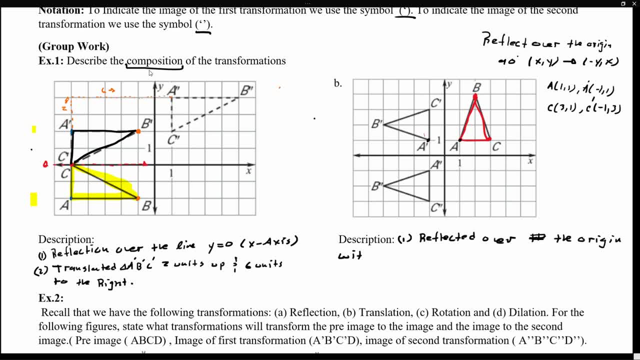 We reflect that over the origin With an angle of rotation Of 90 degrees. So that's the first thing that we did. We got A And we rotated 90 degrees. That's all that has happened here. OK, So now we are at A prime, B prime and C prime. 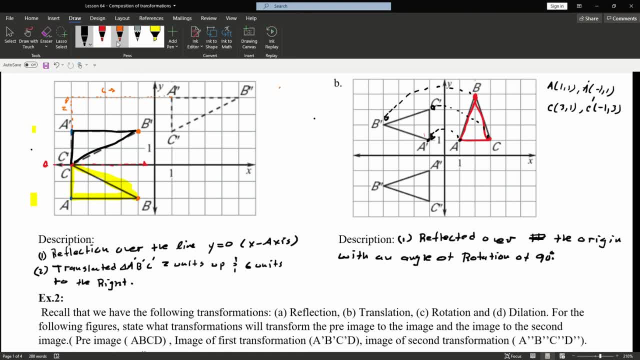 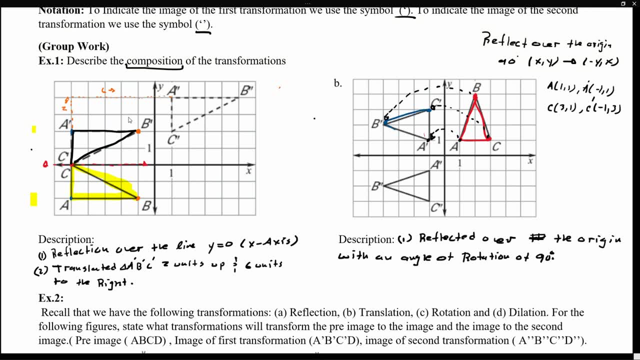 So what exactly can we do to this object? What exactly can we do to A prime, C prime and B prime? So what exactly can we do to this triangle? So it maps exactly on the triangle below, So notice that A should get landed here. 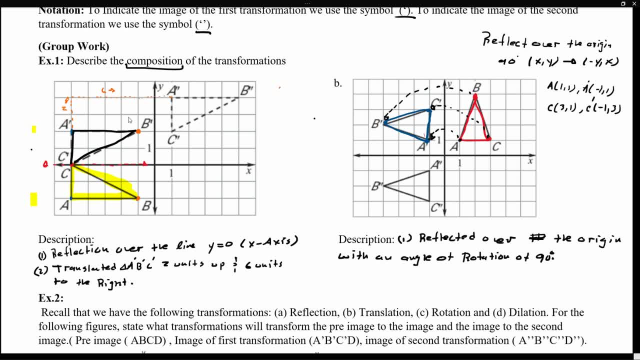 C should get landed here And B should get landed here, But notice that A is one unit away from the x-axis And A prime is one unit away from the x-axis as well. C prime is three units away And C double prime is three units away. 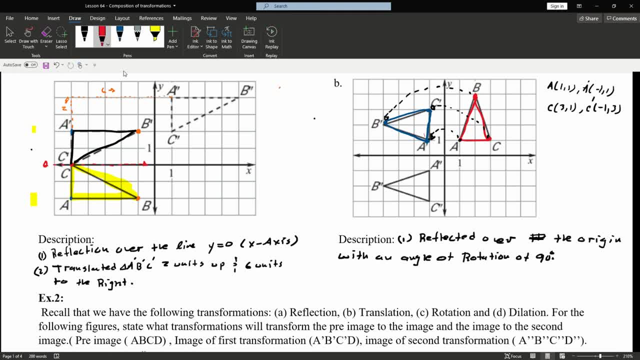 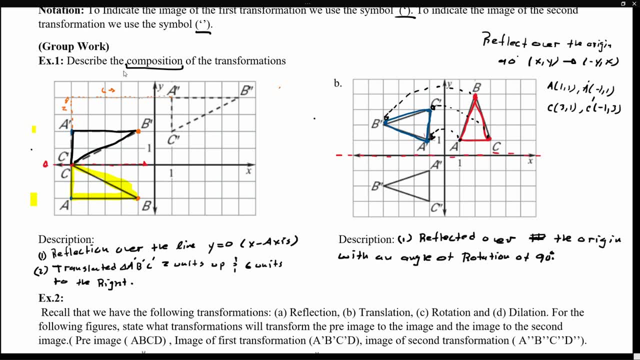 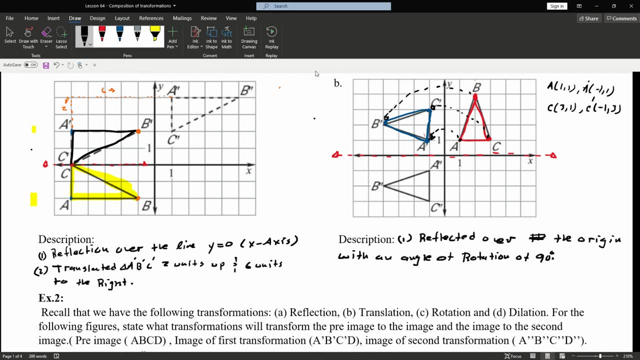 So you can start seeing that this will be an example of a reflection Still over the x-axis. This will be an example of a reflection over the x-axis. So the first thing that we did, we reflected over the origin with an angle of rotation of 90 degrees. 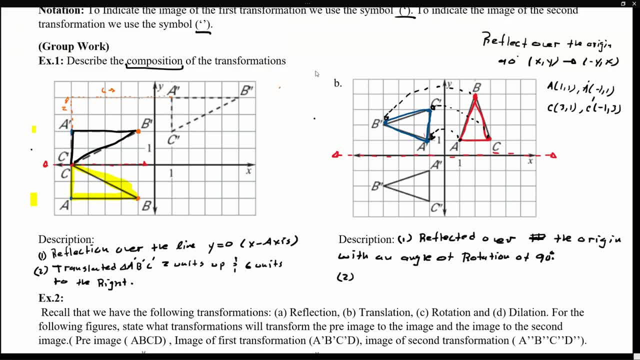 And now, in order to land A prime C prime, B prime on A double prime B, double prime, C, double prime, what we did after that, we've reflected triangle: A prime, B prime, C prime over the line x equals 0..